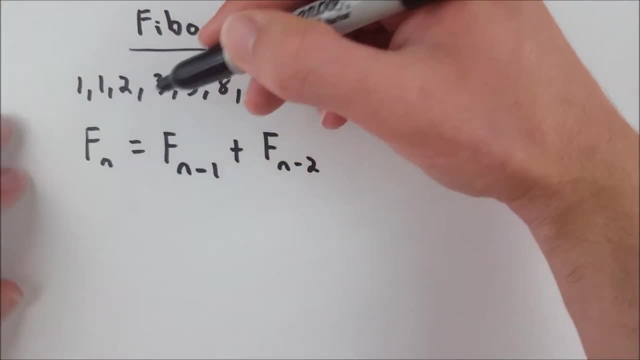 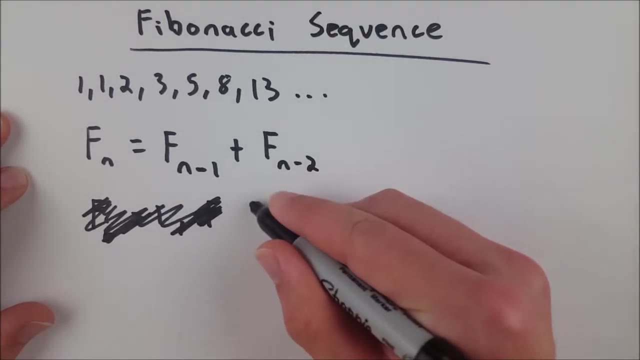 take 5, that's equal to 3 plus 2.. Since this is a second order recurrence relation, we need two initial conditions. Sorry, I didn't like what I was writing in there, so we'll say we have these two initial conditions: F sub 0 equals 1, and F sub 1. 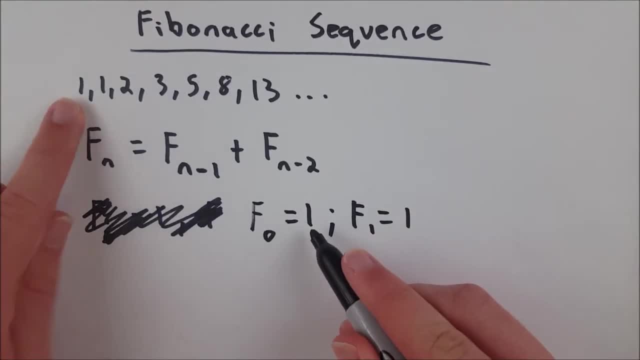 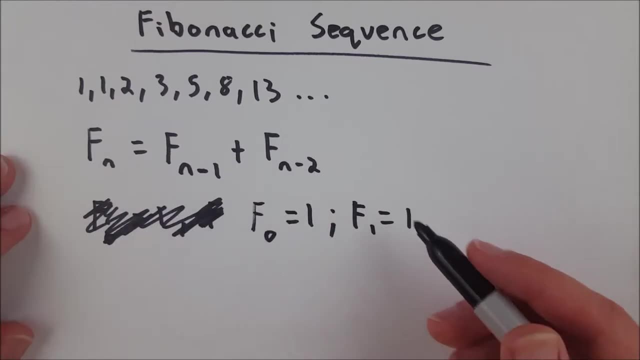 also equals 1, so that gives us this one and this one, And from then on we can figure out every Fibonacci number by taking the sum of the previous two. So when we define this recurrence relation, we'd also say that n is greater than or. 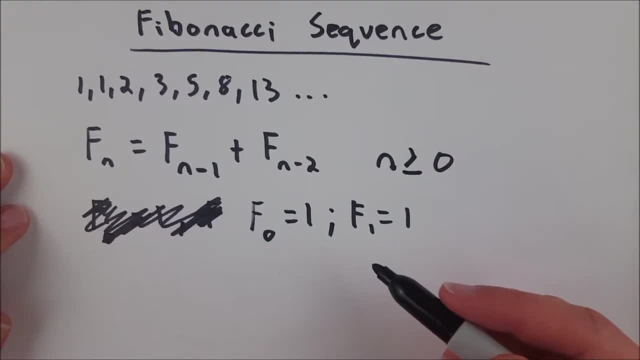 equal to zero. Those are the only ends we're working with, of course. If n equals zero, then our number is one, If n equals one, our number is one, and from then on we can use this relation right here Now. sometimes the Fibonacci sequence is started with a zero, and so in that case it's. 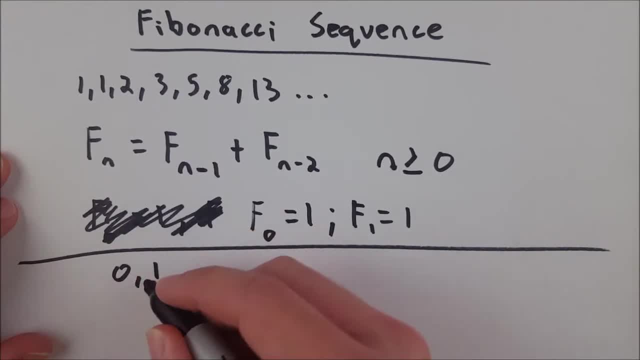 very similar, but it looks like this: Zero one, and then you add the two previous numbers to get one, and then two, and then so on. You're right back into the sequence as it appears above, And that's really all there is to it. Just to show you an example of using this recurrence relation: 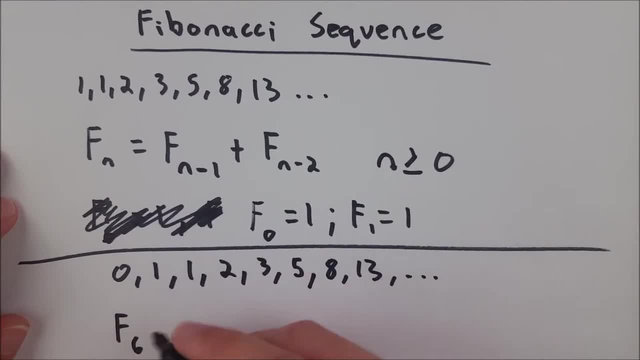 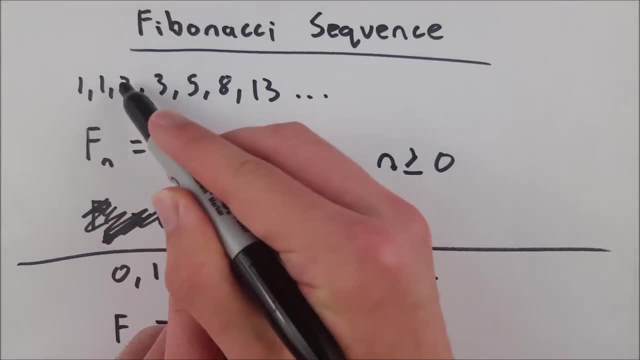 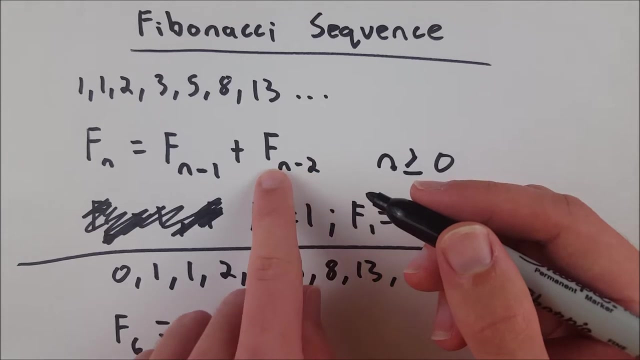 let's say we want to find out what the sixth Fibonacci number is. So we'll take the fifth Fibonacci number- Six minus one is five. One, two, three, four, five, That's five- and add to it the fourth Fibonacci number. Six minus two is four. One, two, three, four That's three, So the sixth. 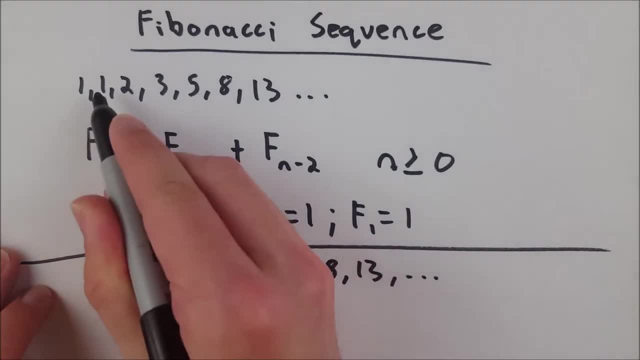 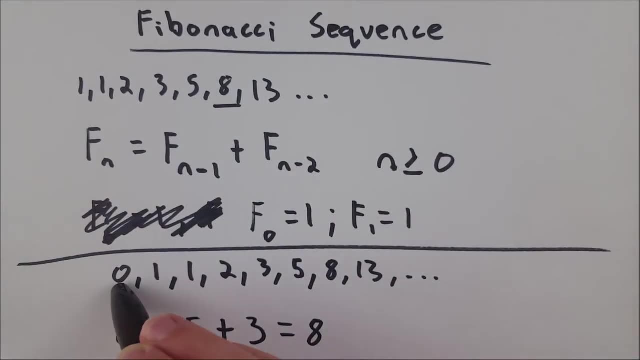 Fibonacci number is five plus three, which equals eight. One, two, three, four, five, six. There's our eight Checks out just fine, And of course it would be just about the same thing if we started with zero, but you're basically just shifting the whole. 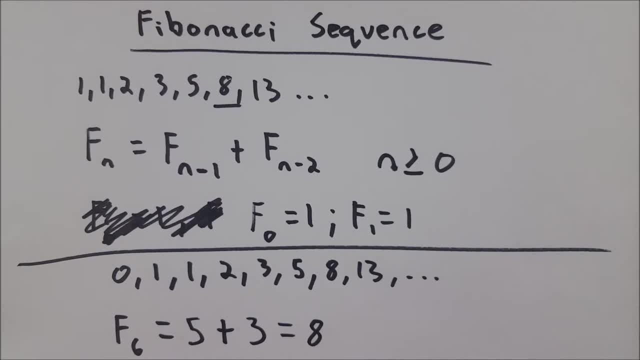 sequence, up one and adding in that additional number right at the start. So that's what the Fibonacci sequence is. It's a sequence of numbers where, after the first two numbers, every subsequent number is defined as being the sum of the previous two. So I hope this video helped you understand. 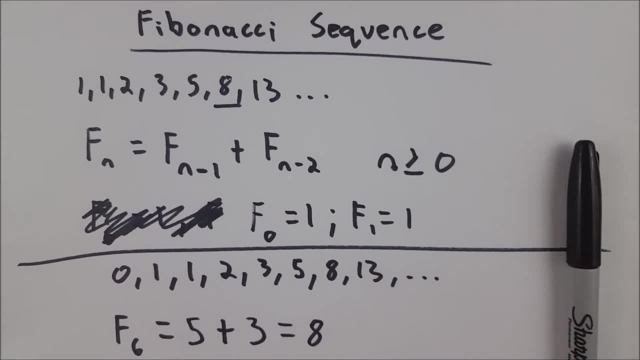 what the Fibonacci sequence is and how we can write it as a recurrence. Let me know in the comments if you have any questions, if you need anything clarified or if you have any other video requests. Thank you very much for watching. I'll see you next time and be sure to subscribe for the swankiest math videos on the internet.